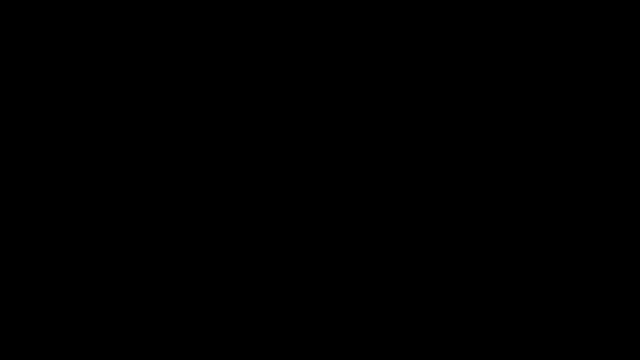 In this video I want to talk about how we can convert repeating decimals into fractions. So let's give ourselves a repeating decimal. So let's say I had the repeating decimal 0.7, and sometimes it'll be written like that, which just means that the 7 keeps on repeating. 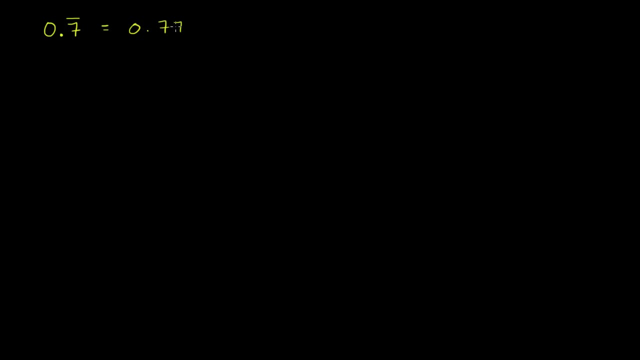 So this is the same thing as 0.7777, and I could just keep going on and on and on forever with those 7s. So the trick to converting these things into fractions is to essentially set this equal to a variable, And we'll just show it. do it step by step. 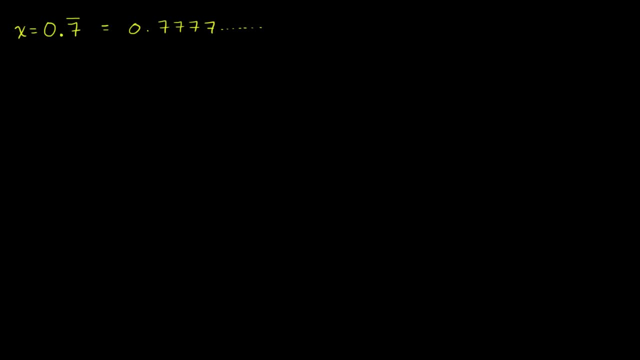 So let me set this equal to a variable. Let me call this x, So x is equal to 0.7, and then the 7 repeats on and on forever. Now, what would 10x be? Well, let's think about this. 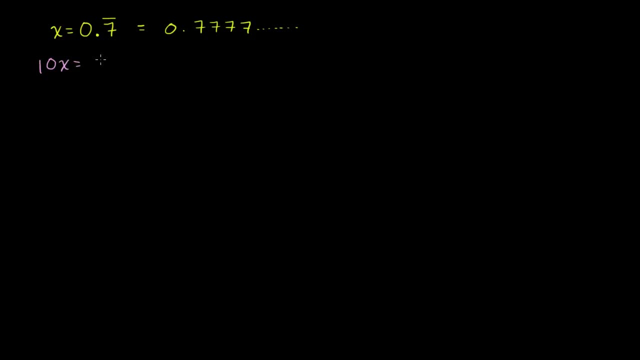 10x would just be 10 times this. So it would be- and we could even think of it right over here- it would be if we multiplied this times 10, you'd be moving the decimal 1 over to the right. 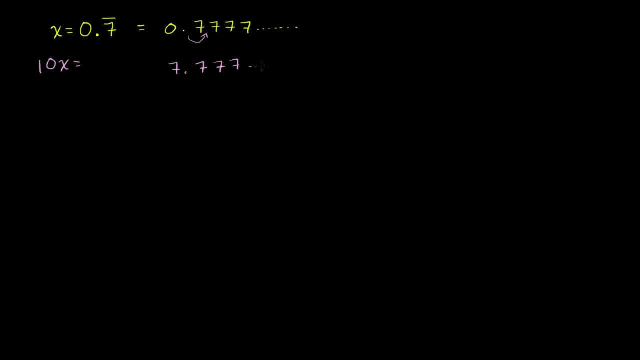 It would be 7.777, on and on, and on and on forever. Or you could say it is 7.7, repeating. Now this is the trick here, So let me make these equal to each other, So we know what x is. 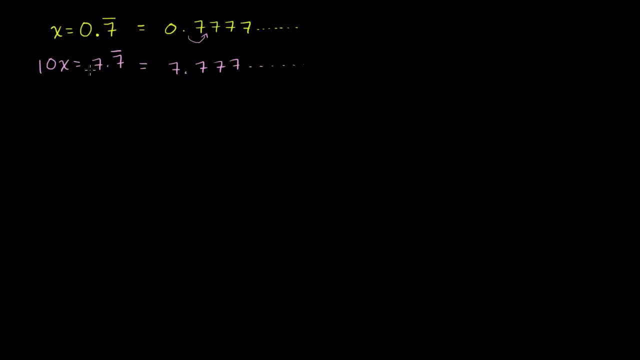 x is this, this 0.777, repeating forever. 10x is this, and this is another repeating thing. Now, the way that we can get rid of the repeating decimals is if we subtract x from 10x, right, Because x has all these 0.7777.. 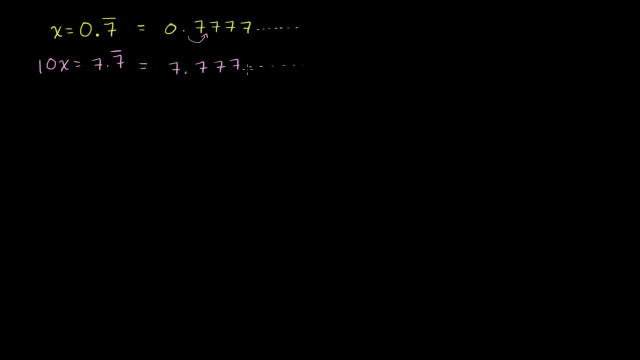 If you subtract that from 7.7777, then you're just going to be left with 7.. So let's do that. So let me rewrite it here, just so it's a little bit neater: 10x is equal to 7.7, repeating which: 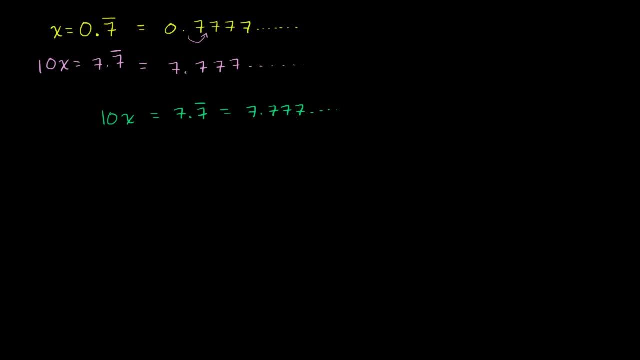 is equal to 7.777, on and on forever. And we established earlier that x is equal to 0.7, repeating which is equal to 0.777, on and on forever. Now what happens if you subtract x from 10x? 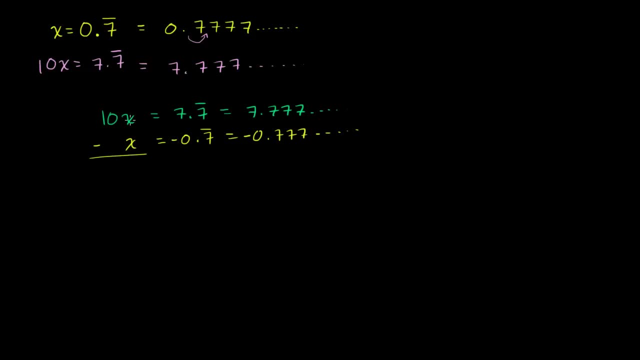 So we're going to subtract the yellow from the green. Well, 10 of something minus 1 of something is just going to be 9 of that something, And then that's going to be equal to what's 7.7777 repeating minus 0.7777, going on and on forever. 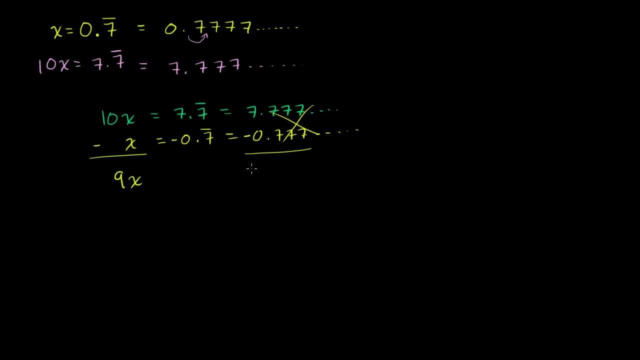 repeating: Well, it's just going to be 7.. These parts are going to cancel out. You're just left with 7.. Or you could say: these two parts cancel out, You are just left with 7.. And so you get: 9x is equal to 7.. 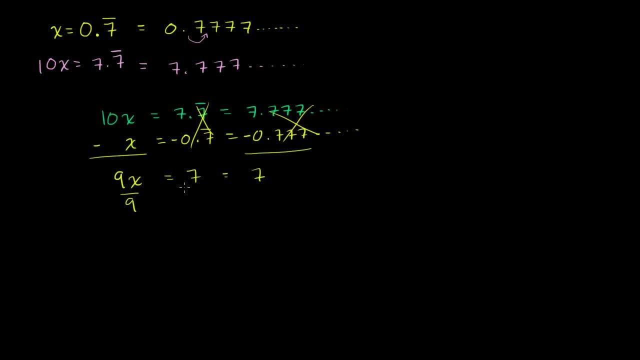 To solve for x, you just divide both sides by 9.. Well, I could do all three sides, although these are really saying the same thing, And you get: x is equal to 7 ninths. Let's do another one. I'll leave this one here so you can refer to it. 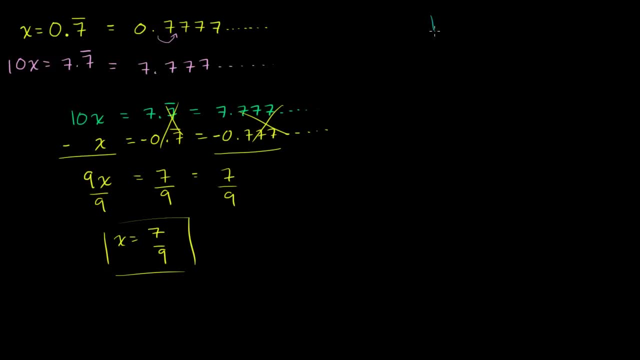 So let's say I have the number 1.2 repeating. So this is the same thing. This thing is 1.2222. on and on, and on. Whatever the bar is on top of that's the part that repeats, on and on forever. 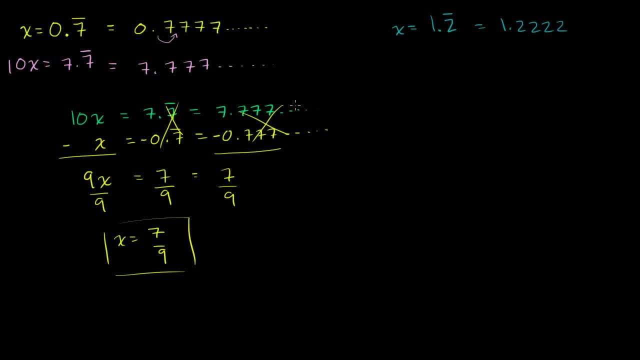 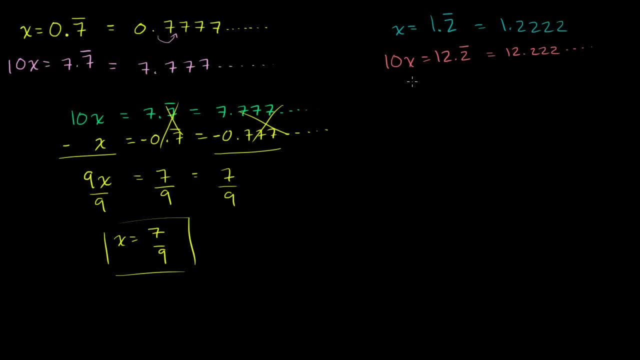 And then we can subtract x from 10x And you don't have to rewrite, But I'll rewrite it here, just so we don't get confused. So we have: x is equal to 1.2 repeating. And so if we subtract x from 10x, what do we get? 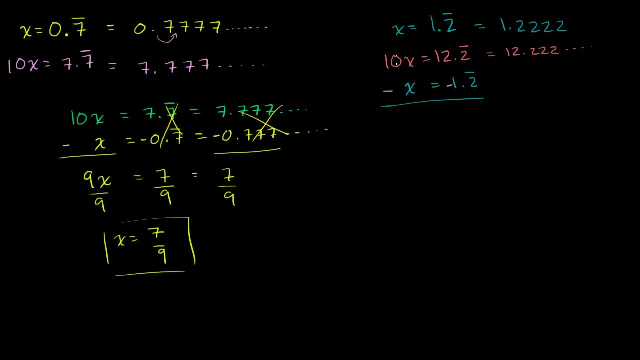 On the left-hand side we get 10x minus x is 9x And this is going to be equal to well. the two repeating parts cancel out. This. cancels with that If 2 repeating minus 2 repeating. 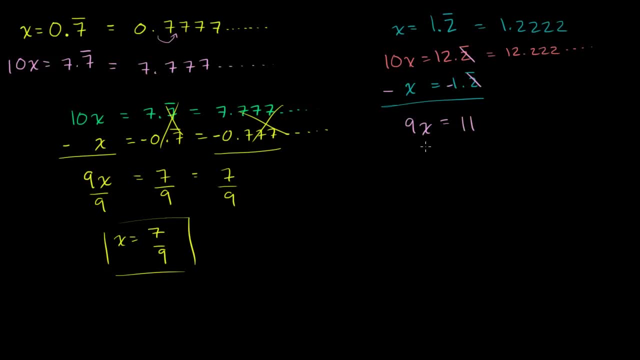 that's just a bunch of 0's. So it's 12 minus 1 is 11.. You have 9x is equal to 11.. Divide both sides by 11.. OK, So by 9, you get x is equal to 11 over 9..